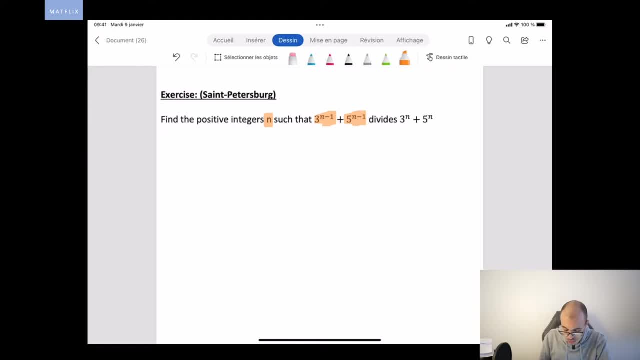 5 to n-1 divides 3 to n plus 5 to n power. So let's try to find these integers, these positive integers, Correction. So actually, here, actually, we have to notice something very interesting. We notice that we notice here that 3 to n plus 5 to n actually is between 3 times 3 to n minus 1 plus 5 n minus 1.. 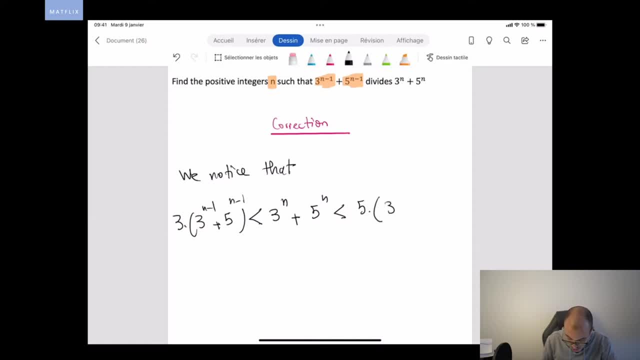 And 5 times 3 to n minus 1 plus 5 to n minus 1.. Why? Because you have, we have here 3 to n minus 1, is is 3, actually is less than 5, and if we, if we multiply each side by 3 to n minus 1, we will have 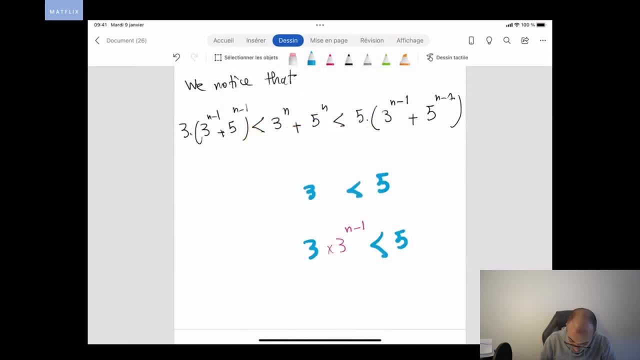 5, and here 3, 3 to n minus 1, and actually that means that 3 to n is less than 5 times 3 to n minus 1, and if we add 5, 5 to n, each side- 3 to n plus 5 to n- is less than 5 times 3. 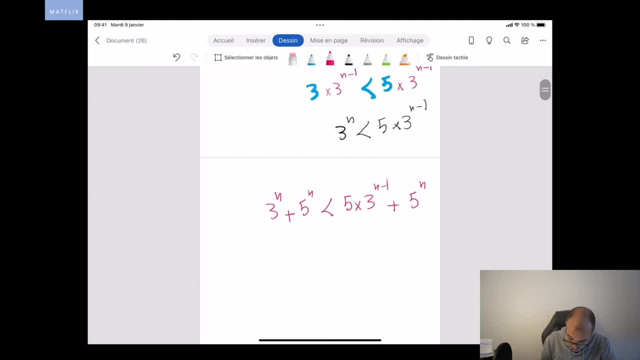 to n minus 1 plus 5 to n. here we can factorize by 5 and we can prove that we have 3 to n plus 5 to n is less than 5 times 3 to n minus 1 plus 5 to n minus 1, and. 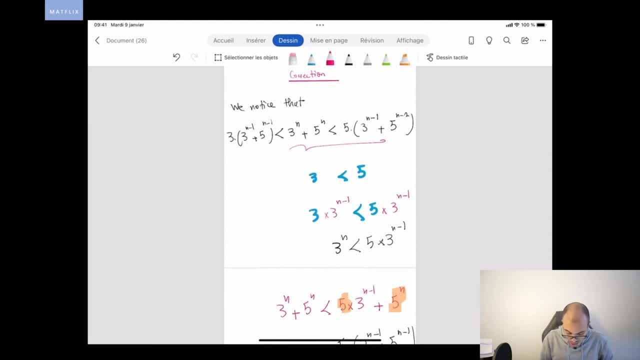 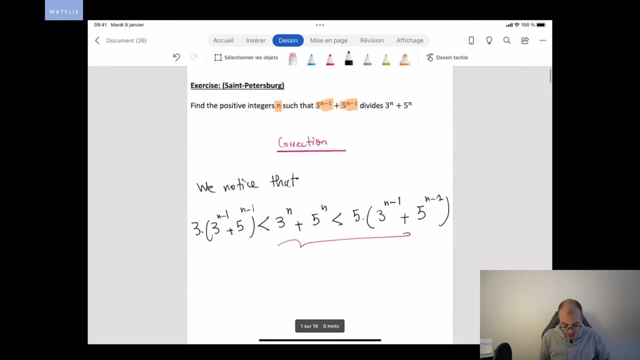 that's how we can prove this inequality. and here we do the same, exactly the same, the other side, and that leads us to conclude that actually, 3 times 3 to n minus 1, plus 5 to n minus 1 is less than 5 times 3 to n minus 1, plus 5 to n minus 1. 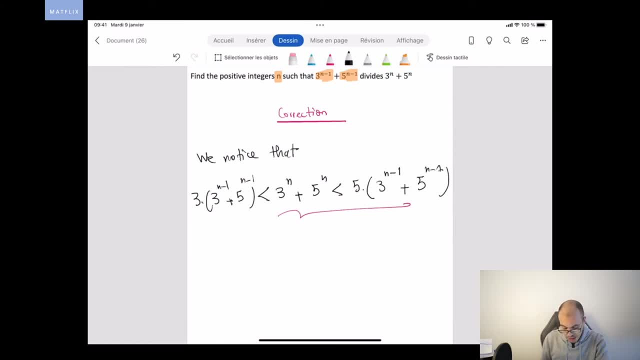 is less to less than 3 to n plus 5 to n. it's exactly the same, the same method. so here we have this double inequality. we can, so we can deduce that 3 to n plus 5 to n if we divide by 3 to n minus 1, plus 5 to n minus 1, we are between 3 and 5 actually. so here we. 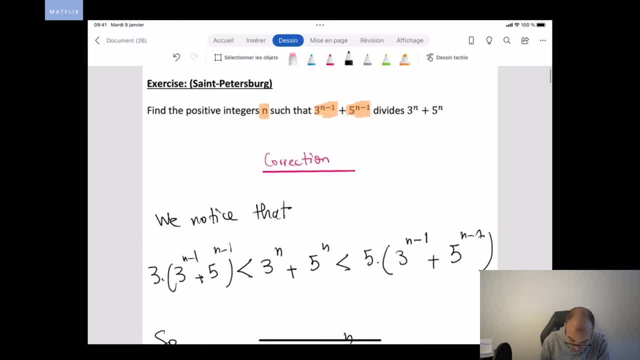 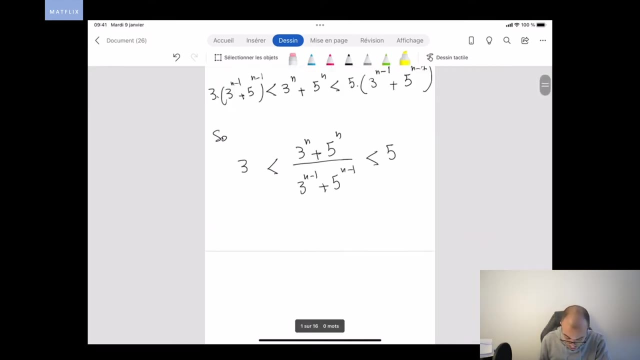 were looking for positive integers n that satisfy. 3 to n minus 1 divides 3 to n plus 5 to n. so this fraction have to has to be an integer. so if 3 to n plus 5 to n divides 3, sorry, if 3 to n minus 1 plus 5 to n. 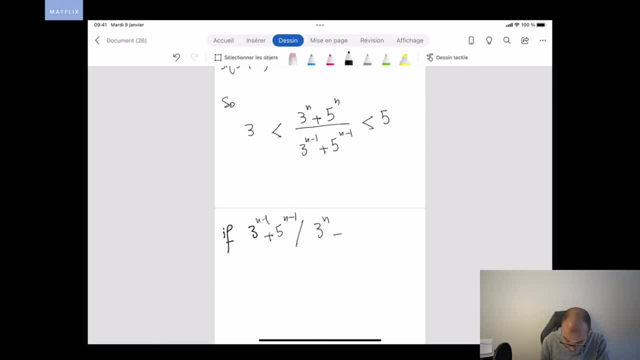 minus 1 divides 3 to n plus 5 to n power. 3 to n plus 5 to n. here over 3 to n minus 1 plus 5 to n minus 1 is integer, and here it must be equal to 4. 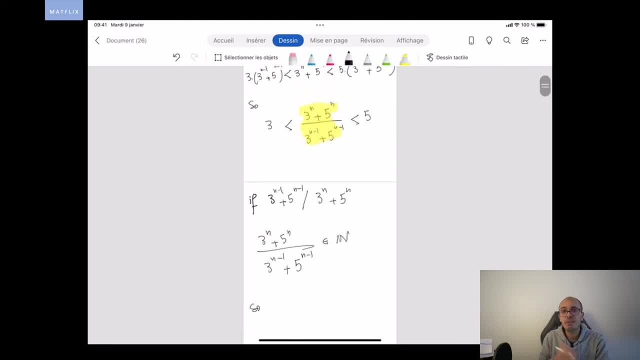 so, as this fraction is between 3 and 5, the only solution is that 3 to n plus 5 to n over 3 to n minus 1 plus 5 to n minus 1 must be equal to 4, because the only integer between 3 and 5 is 4. we can deduce that: 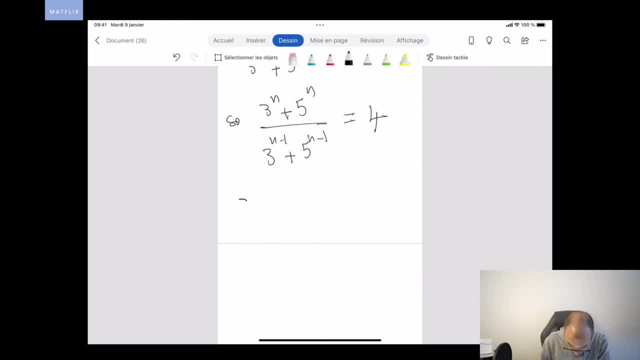 then 3 to n plus 5 to n is equal to 4 times 3 to n plus 5 to n minus 1 plus 4 times 5 to n minus 1. okay, but here 4 is 3 plus 1 times 3 to n minus 1. 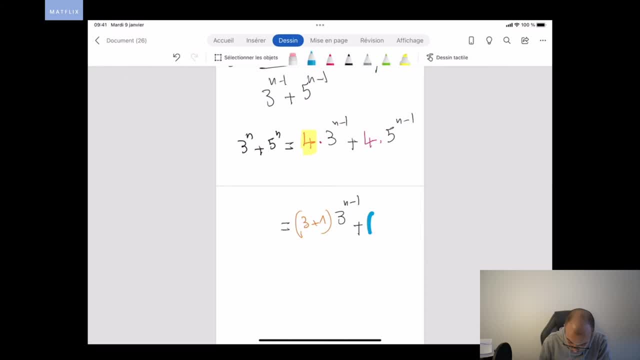 and 4. we can write 4 as 5 minus 1 times 5 to n minus 1. if we develop here, we have 3 to n plus 3 to n minus 1 plus 5 to n minus 5 to n minus 1, and this is equal to 3 to n plus 5 to n power. 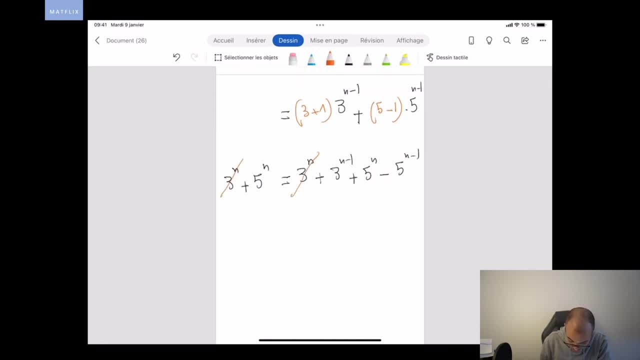 we can here simplify: 3 to n and 5 to n, and this is equivalent to 3 to n minus 1 to 3 times n minus 1, equal to 5 to n minus 1, if we, uh, if we write it like that. so. 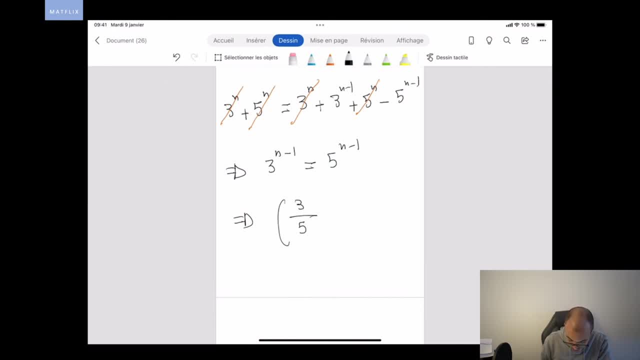 it means that 3 over 5 to n minus 1 is equal to 1. okay, and that means that the power here is 0. so n minus 1 is equal to 0. so n is equal to 3.. is necessary equals to 1.. So the only positive integer, n that satisfies. 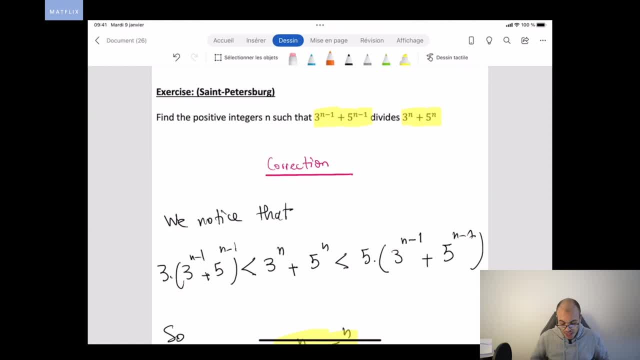 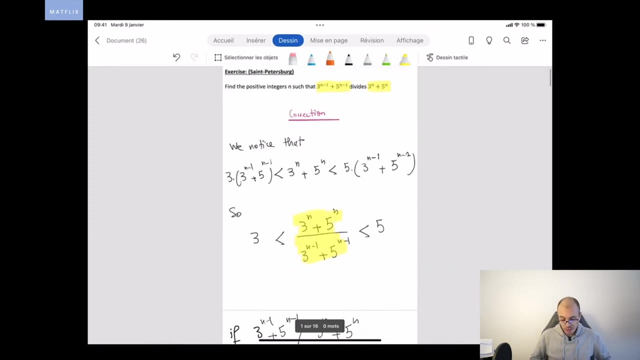 that, such that 3 to n minus 1 plus 5 to n minus 1, divides 3 to n plus 5 to n is 1, and that was the methodology to resolve this exercise, As you. as you notice, here we didn't use any of complex theorems, so tell me in the comments if 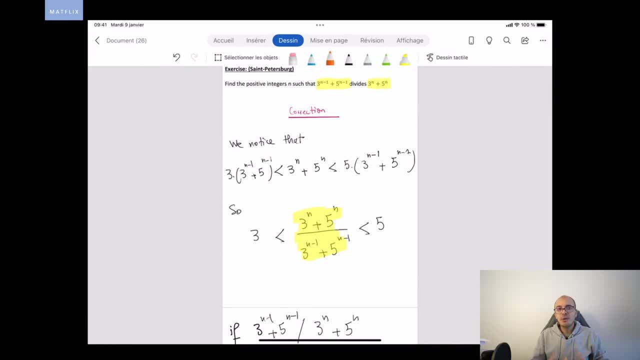 you found. you found the same methodology as as mine, and don't forget to subscribe to this channel, to comment, to like to share. don't forget to hit the bell in order to get notified whenever I post and see you in the the next video.